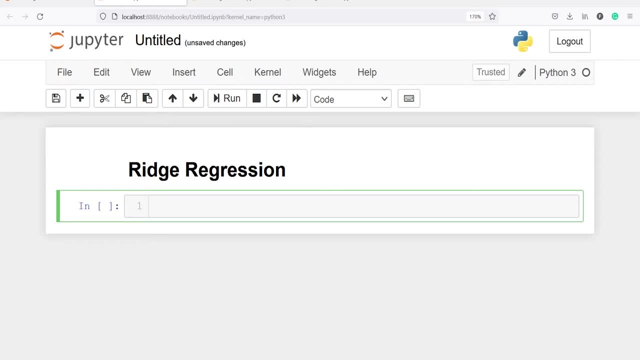 In this video, you will learn about rich regression. Rich regression is used to create a simple model when the number of independent variables are more than the number of samples, or when the data set has multicollinearity, that is, correlation between independent variables. It has a parameter lambda. 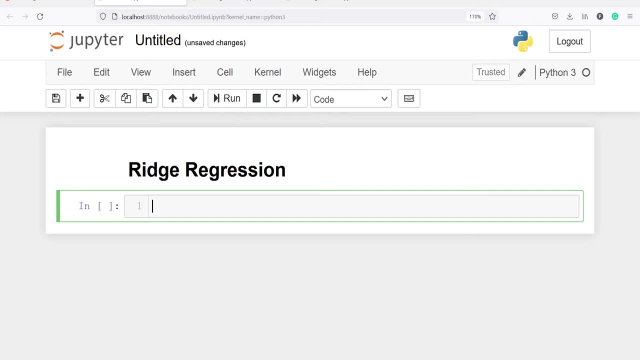 denoted by alpha is known as the penalty term. It helps to reduce the magnitude of coefficients of our independent variables. By changing the values of alpha we control the penalty. Higher the values of alpha, bigger is the penalty and therefore the magnitude of coefficients are. 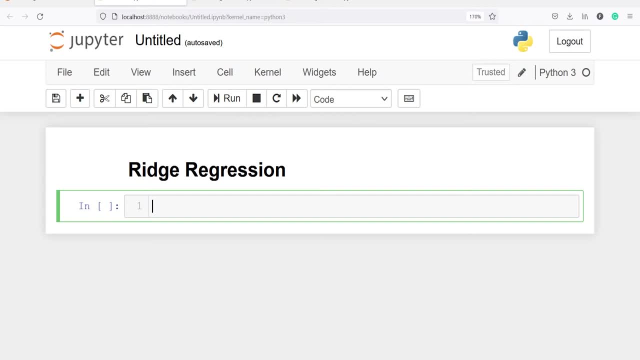 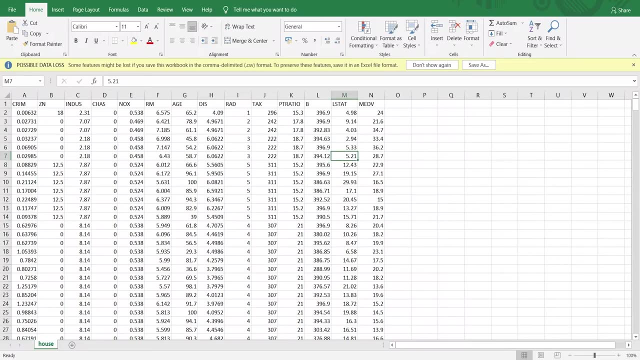 reduced. It uses L2 technique. We will work on housing data set which contains information about the houses in the suburbs of Boston. This is our data set here There are total 506 samples and 14 columns. The goal is to predict the median value of the house. 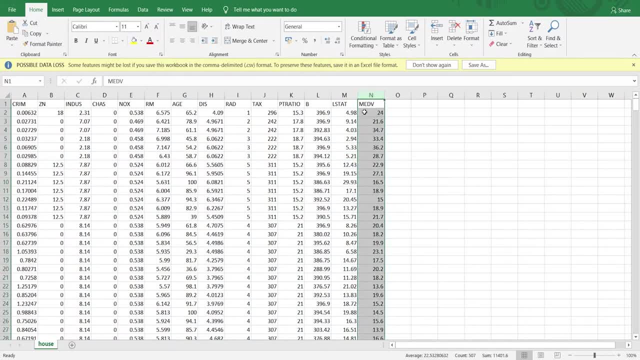 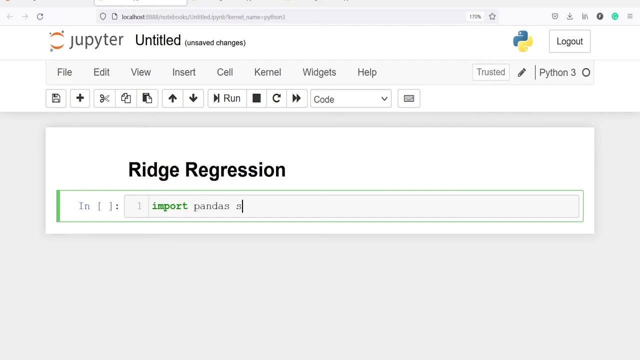 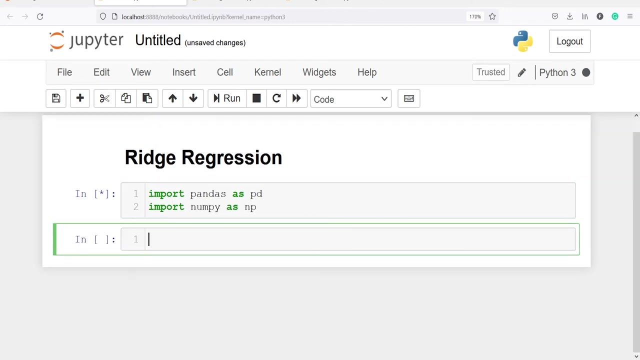 This is the target column MADV. MADV is the target variable. that is the variable that we want to predict using our independent variables. Let's go to Jupyter notebook and import our data. Let's import Pandas as PD, Import NumPy as Np. I am going to make one variable, DF, From pandas. I will call read. 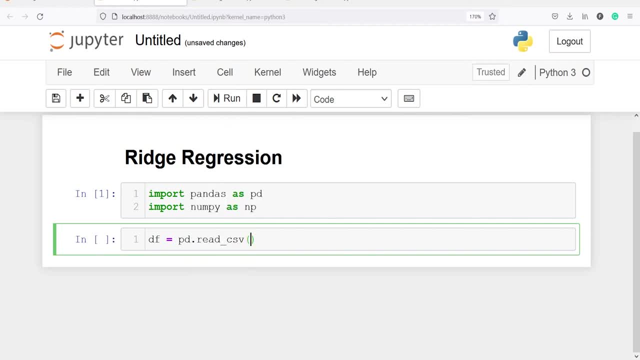 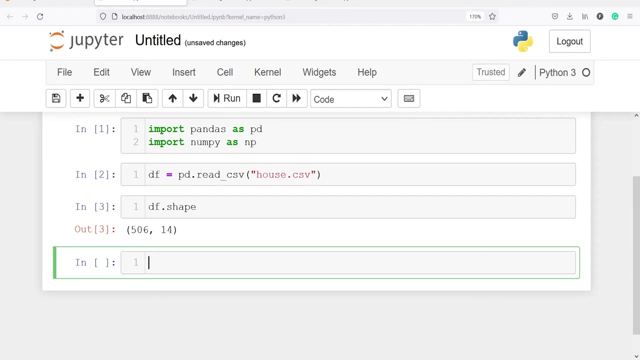 underscore CSV and I will pass my CSV file name: house dot CSV. now let's look at the shape of our data frame. I'll write DF dot shape and we have total 506 rows and 14 columns. we can also check the size of our data frame. we will write DF dot size. 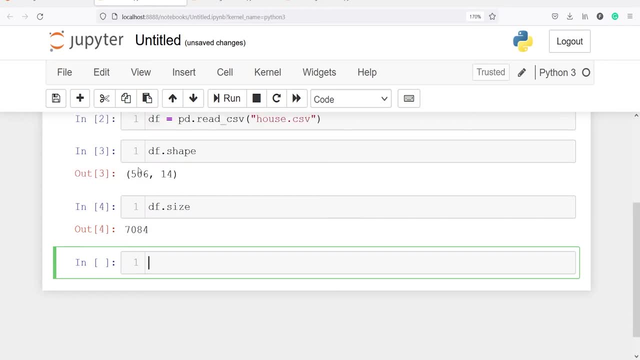 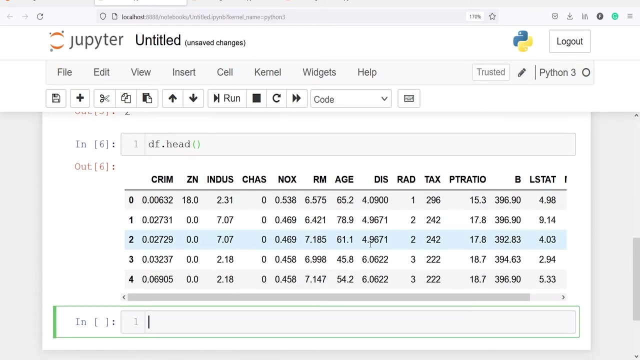 size is 7084. it is multiplication of rows into columns. let's also check the dimensions: DF, dot ending, and it has two dimensions because we have rows and columns. let's look at the top five rows of a data frame. we will use the method head, DF, dot head. these are the top five rows of a data frame and we have columns. 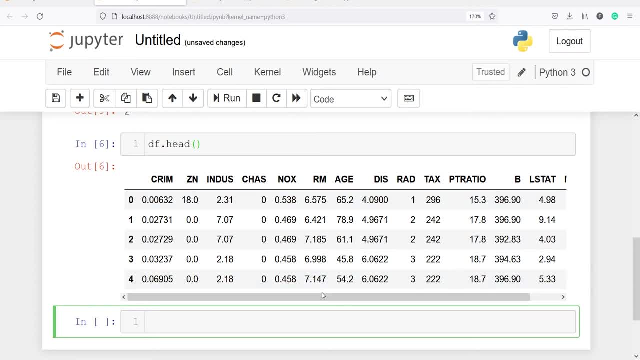 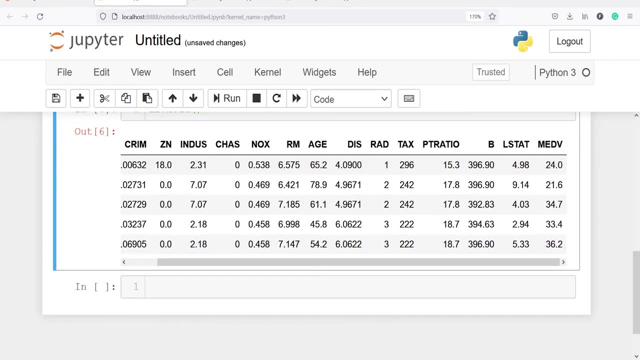 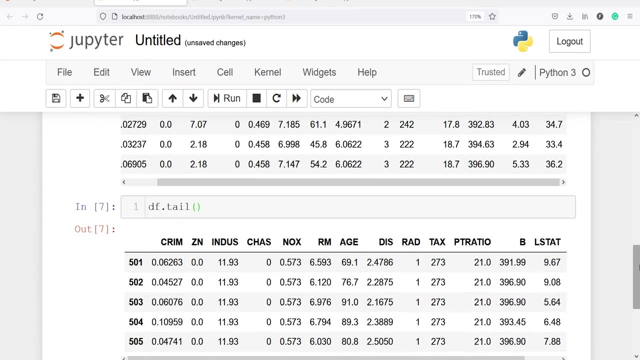 such as C R I M Z, N, I, N D U S and so on. we have a column M, E, D V. this is our target variable. let's look at the bottom five rows of a data frame. using the method tail, we will write DF dot tail, and these are the bottom five rows of a data frame. we 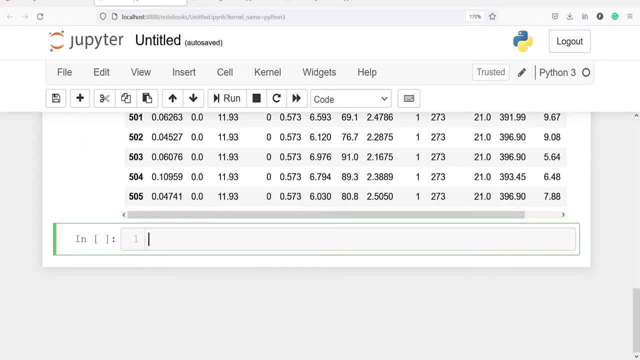 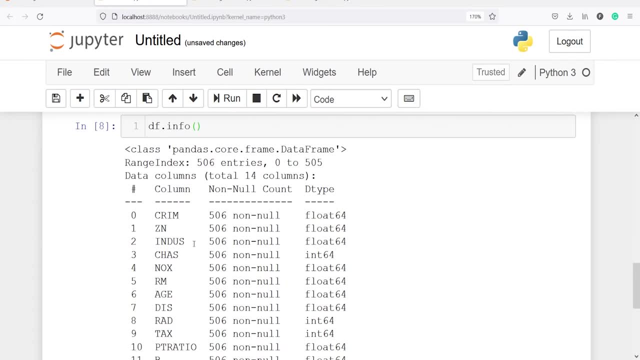 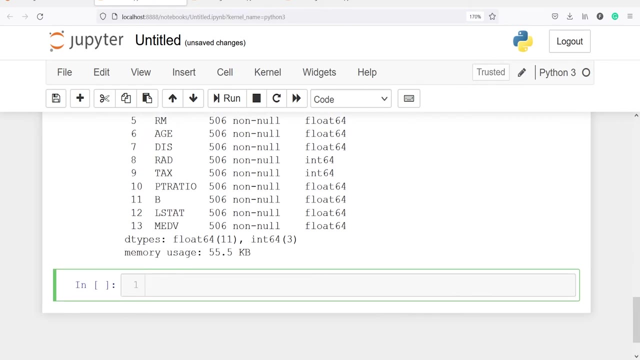 can also get other information using the method info. we will write DF dot info and here in the output we will get some information such as the column, name, non null count and the data type of each and every variable. we can also get the descriptive statistics using the method describe. we will write DF dot describe. I'll write DF dot describe. we will write DF dot describe. 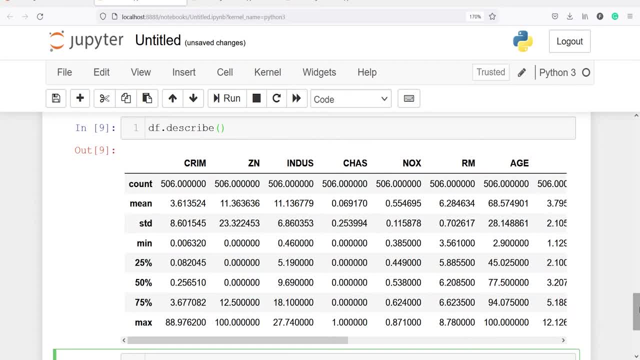 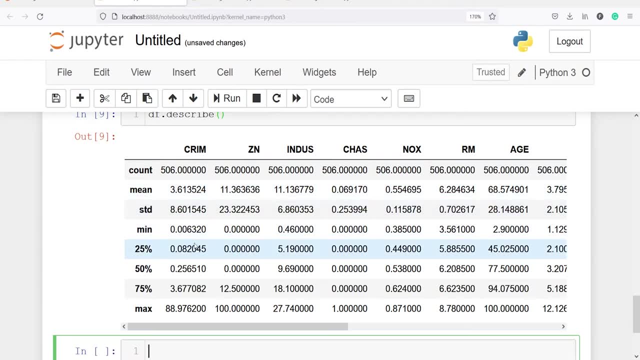 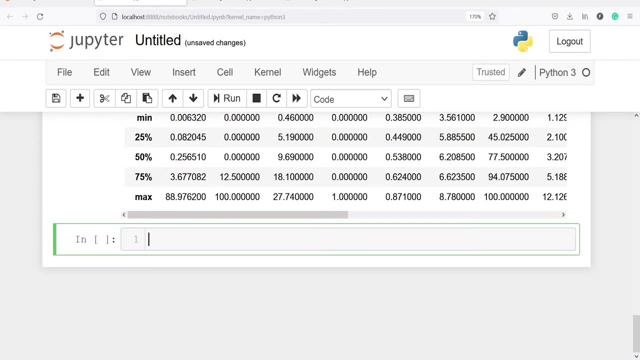 in the output you can see we got the descriptive statistics and we have such as count, mean, standard deviation, minimum, 25%, 50%, 75 percent and maximum. if you want to check the data types, we will use the method D. types. we will write DF dot. 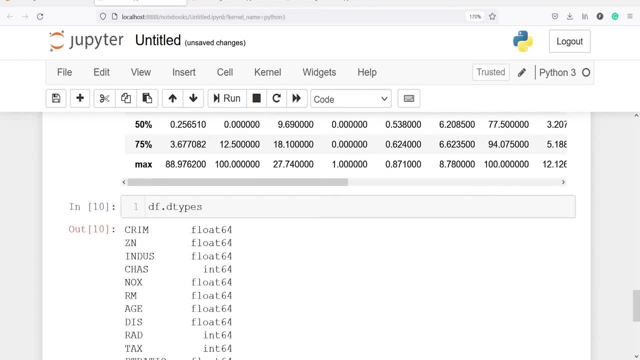 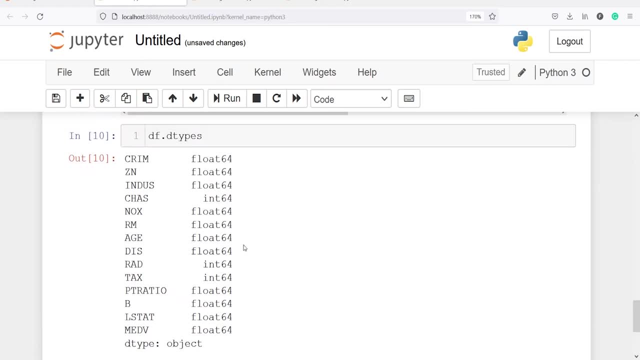 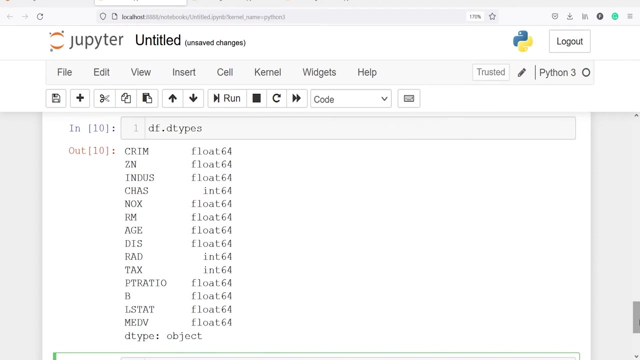 D types and here you will get the column and the data types. so for this column, for example, age, it is 464. so this is how you can get the data types of each and every column. also, we can also check if there are any missing value present in our 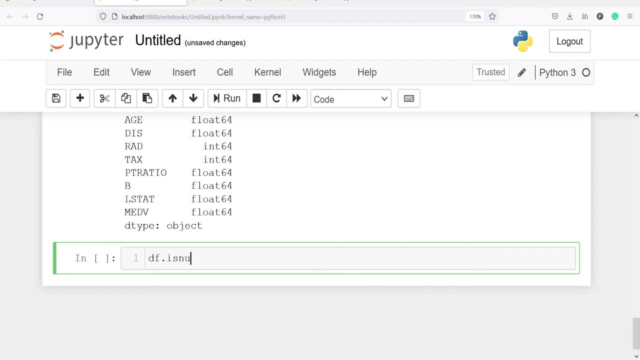 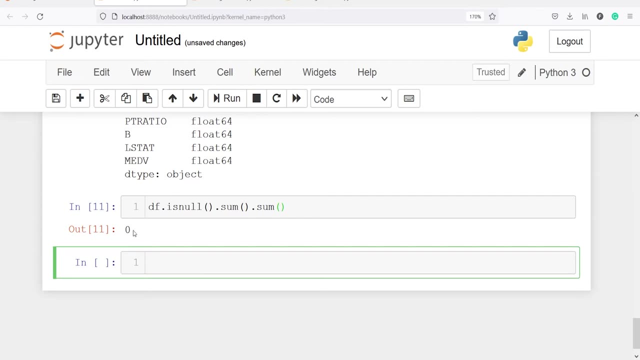 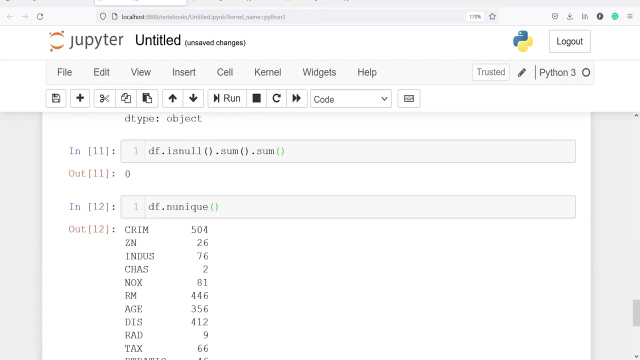 data frame we will write df, dot is null, dot, sum, dot, sum. and here you will see we got zero here, because there are no missing values in our data frame. we can also check if there are unique values present in our columns and we will find that using the method n unique. and here in the output we will see we got some. 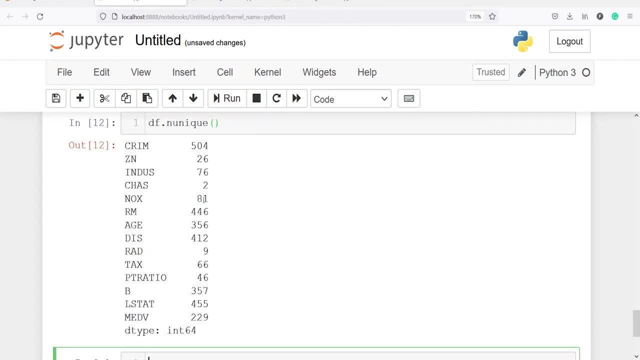 numbers. here, for example, 81, so there are 81 unique categories or unique values present in the variable nox. here, age 356, so there are total 356 unique age present in our variable age. next we will find the correlation between variables. I will use the method CORR and here in: 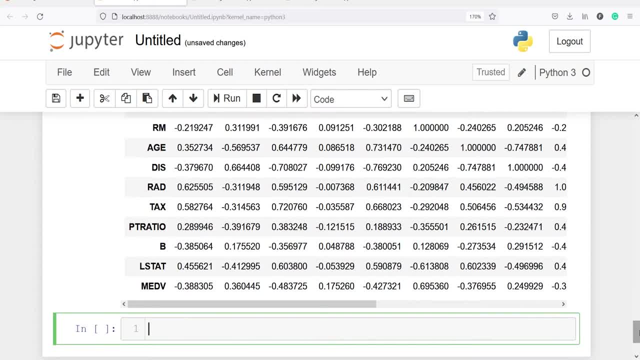 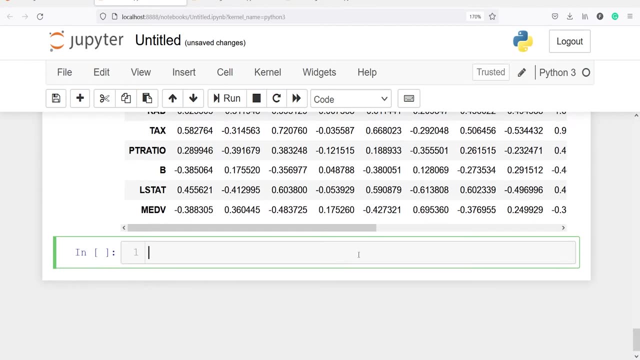 the output we will see. we got the correlation between all the variables and here MADV is a target variable. we can check the correlation with our target variable, for example, if you look here. so the correlation between MADV and CRIM is minus 38 percent. then for the next variable it is 36 percent. for next, 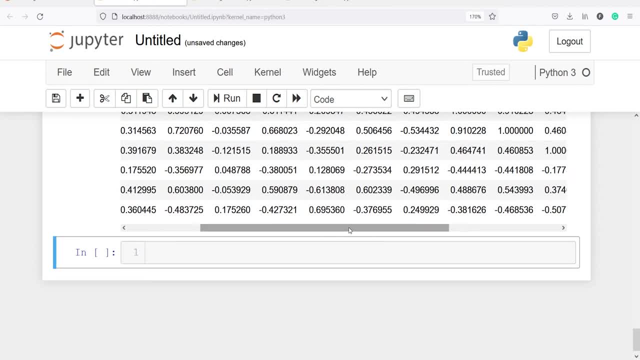 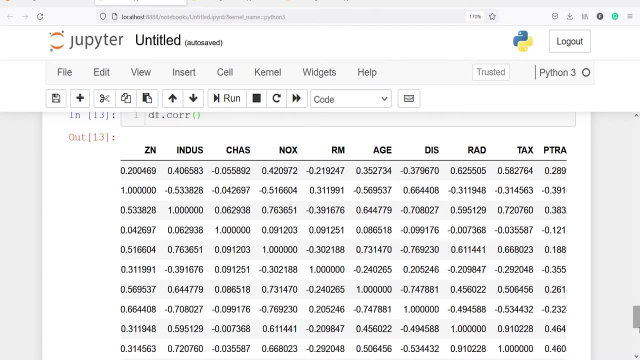 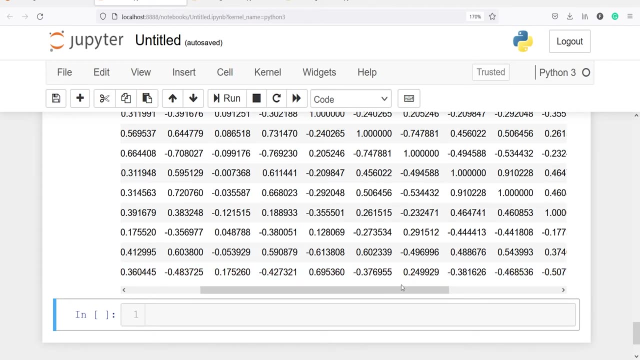 variable. it is minus 48 percent and so on. and here you will see we have this 69% correlation with this variable, RM, which is the highest one. so RM is our most important feature in our model. then we have correlation such as minus 37 percent, minus 24 percent, minus 38 percent, and so on. next we will make the 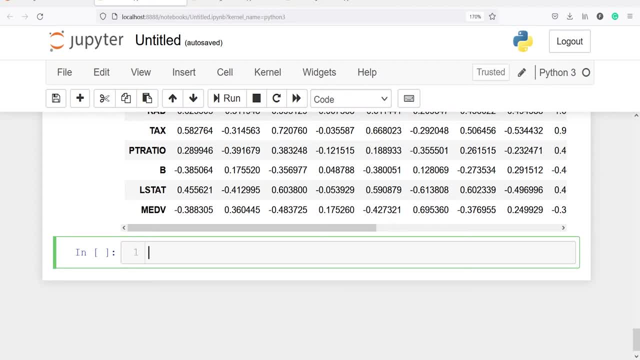 scatter plot. so I will import from import matplotlib dot pyplot as PLT and from ML extend dot plotting. I'll import scatter plot matrix because I'm going to make a scatter plot matrix here now. I'll make one variable column, COLS, and I want to include few columns only, such as first: 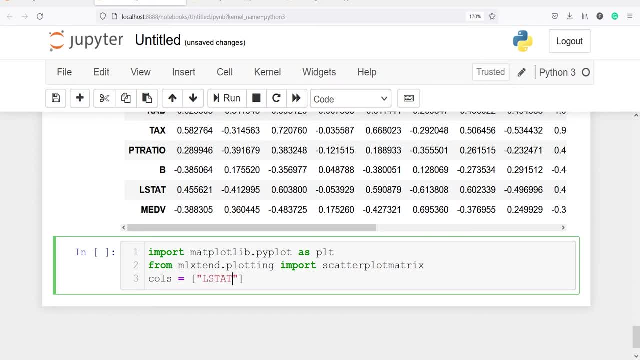 we will include this one, ELSTAT. second is B, third, TAX, TAX, and then our target variable, MADV. next I will call this scatter plot matrix and I will pass our column names. so I will write DF of columns- dot values, because we want to get the values from our data frame. so I'm subsetting DF of columns. 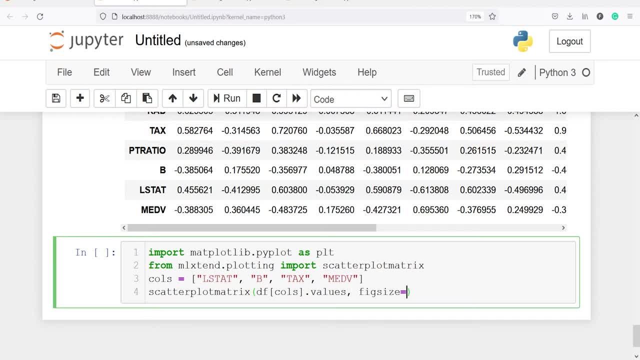 then I will pass on parameter figure size, and it is going to be 10 by 8. next parameter is names. so our names are going to be column names, so I will write COLS. then the next parameter is alpha. it is the transparency of the color. so I am. 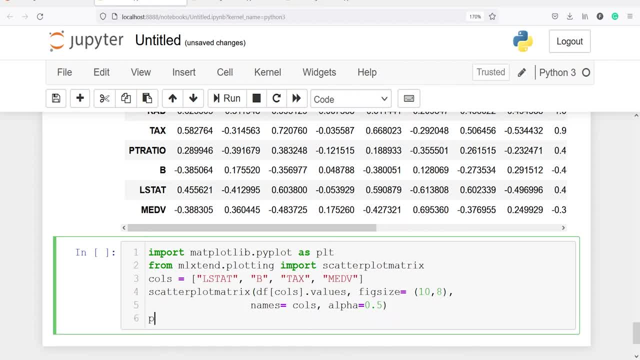 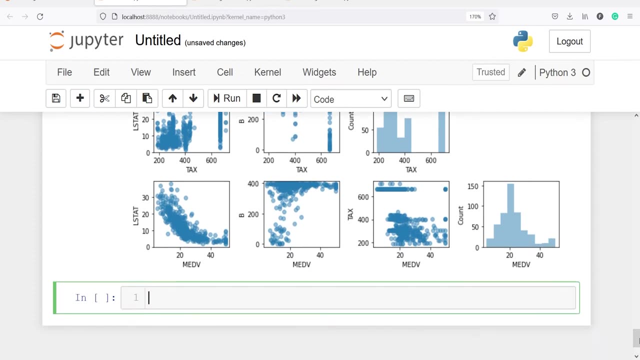 saying it is 0.5, then we will call this parameter alpha, so we will call this. we will call plt dot- tight layout and then finally plt dot- show here in the output. you will see we got the scatter plot here. so this is the scatter matrix, and here we are getting some. 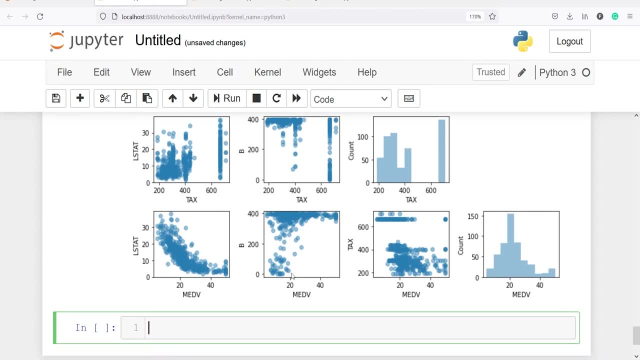 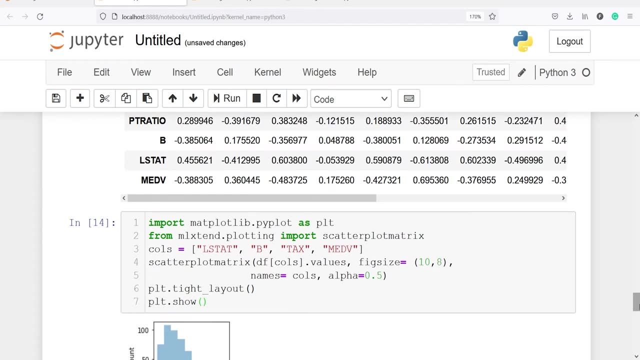 correlation between these independent variable and a target variable, madv, and you will see we don't have any good correlations. but if i put one more variable here, that is rm, and now, if i run it again now you will see that we have a good correlation with rm here. you will see. 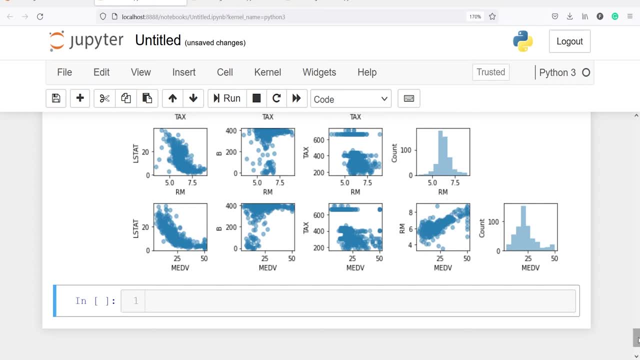 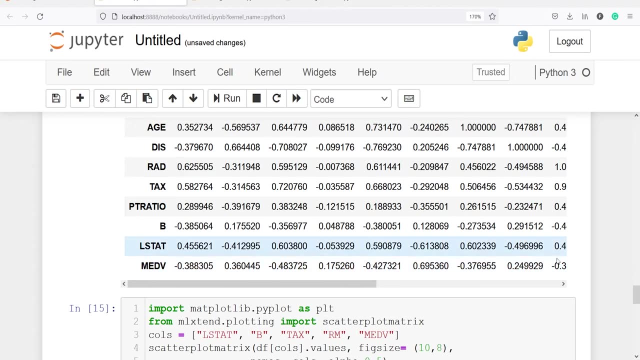 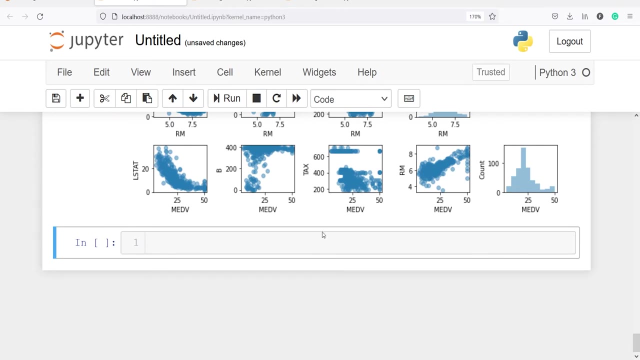 madv and rm. it is going in the same direction because we have already seen about that. the correlation between this rm and madv is 69 percent. so this is the most important feature in our variable. now we are going to make the heat map, so for that i will call from ml extend dot plotting. i will import heat map. 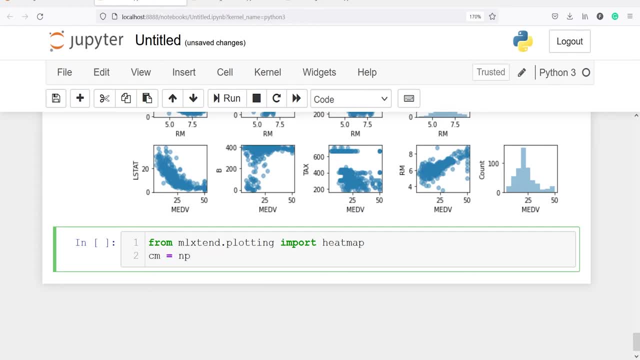 i'll make one variable cm and in this i will save the correlation coefficient and and i will call that using the np, that is, the numpy dot correlation coefficient, this method. using this method we can calculate the correlation coefficient. then we will pass our data frame and we want to get the pollution coefficient of columns. 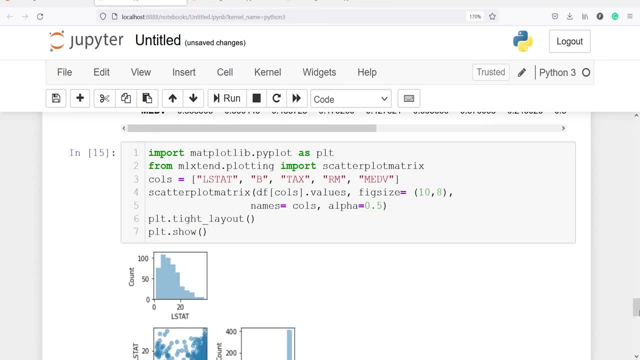 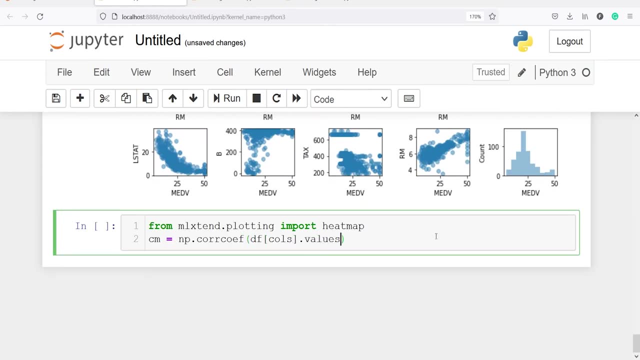 that is all the columns that we have provided above here here in this list. columns here. and to get the values i have to type dot values and i am going to transpose it because i want to get it on the y-axis, so i have typed t here. 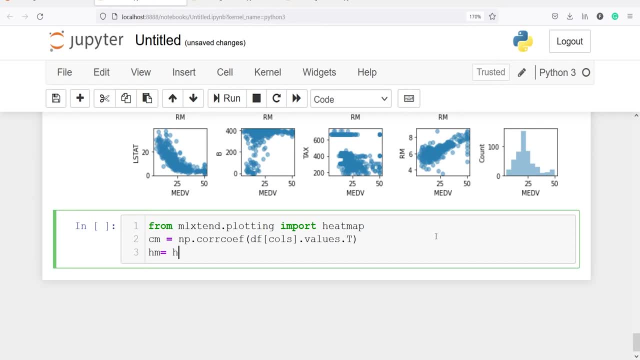 then i'll make one more value, hm, and here i will call the heat map method. inside this i will pass our variable cm that we have saved above here. then i will pass some parameters such as row names. our row names and column names are going to be same, so i have typed columns here, then column names. this is also going. 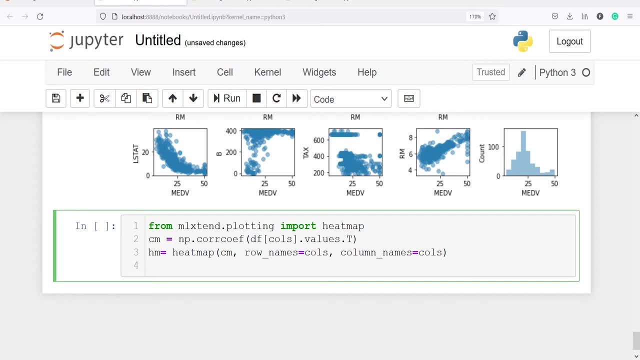 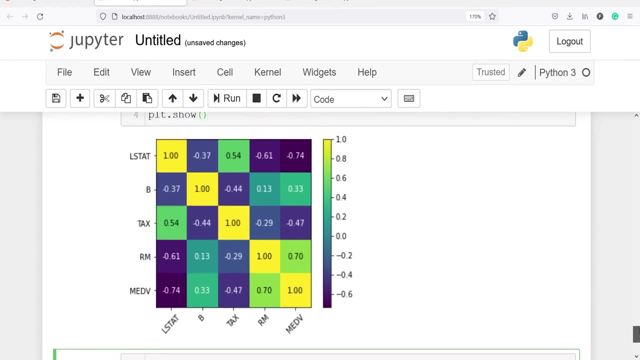 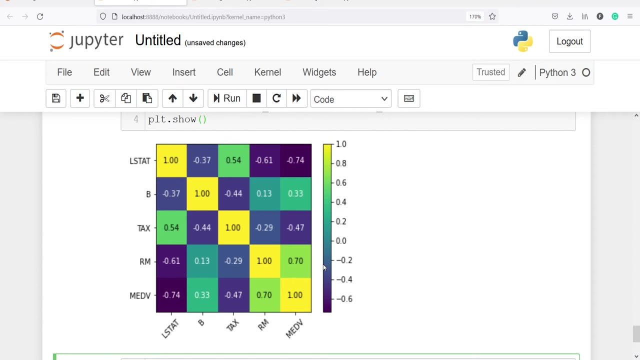 to be same columns. next, plt dot show in the output. you can see we got the heat map here and you will see the correlation between this uh target variable m, a, d, v and r. m is 0.70, that is 70, and for other variables we have correlation such as minus 47 percent, 33 and. 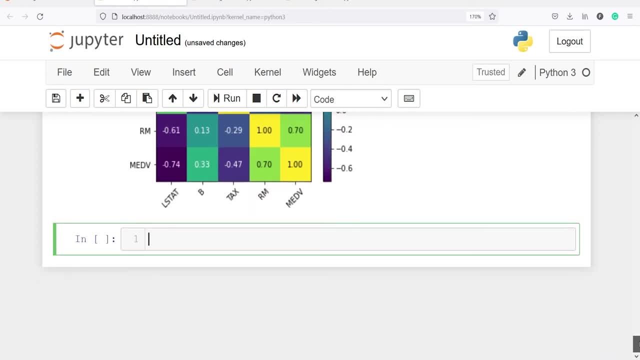 minus 74 percent. we can also plot histogram of our target variable, m, a, d, v, to check the distribution of our data. so i will call pnt, dot, hist and i want to make the histogram of a target variable, df of m, e, d, v, and i'll put the title plt, dot title. the title is going to be histogram. 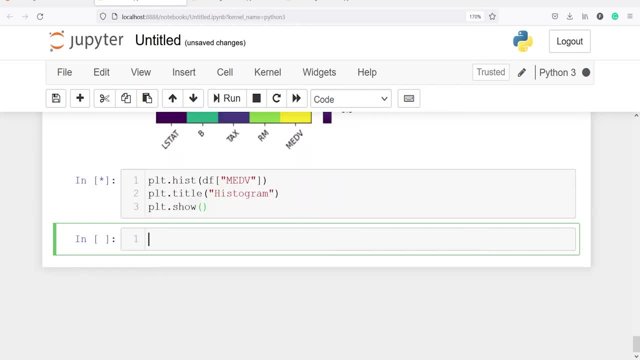 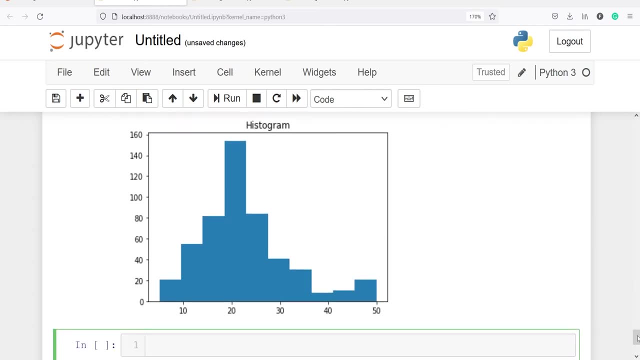 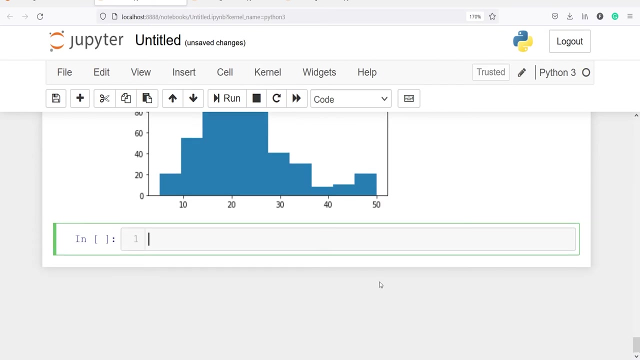 and next plt dot show here in the output. you can see we got the histogram. this will tell us the distribution of our target variable, m, e, d, v. next we are going to split our data frame into x and y variable. in x we will have all the independent variables and in y we will have a target variable. so i'll make x here. 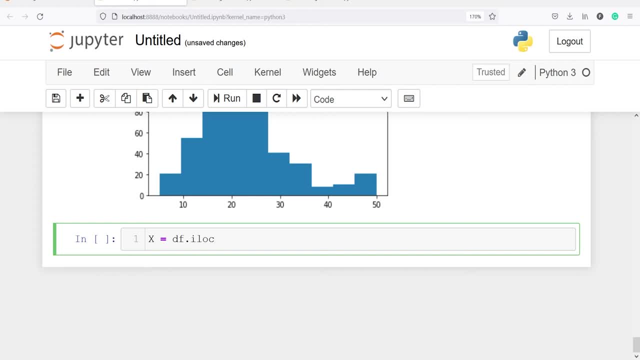 i'll call df, then i will call iloc. i'll make a list. i'll type: colon, column means i want all rows, colon minus one means i want all the column except the last column, because last column is a target variable. then i will make y, df, dot, iloc, and in this i want all column, but i just want the target. 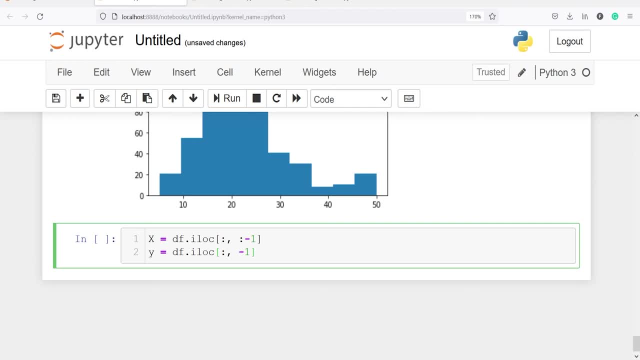 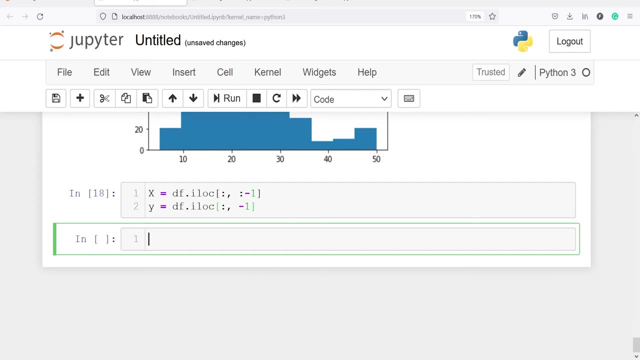 column. so i will write minus one only. let's execute our code. next we will split this x and y into train test, and for that first of all i have to call the train test split from sklearn. so i will write from sklearn dot model selection, import, train test split. then i will make x train. 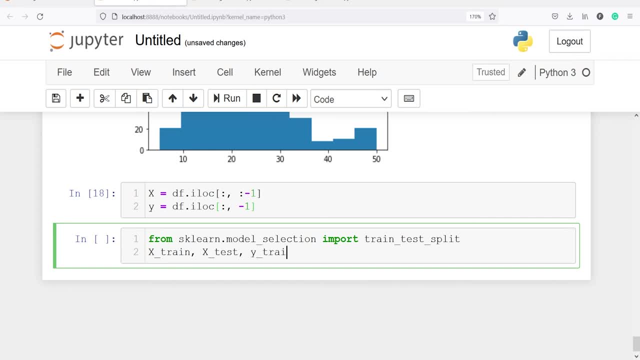 x test, y train y test, train test split. and inside this i will pass x and y and i also pass on parameter random state, and you can put any number here, let's say 10.. if you want your result to be as same as mine, then you have to put 10, otherwise you can put any random number here. 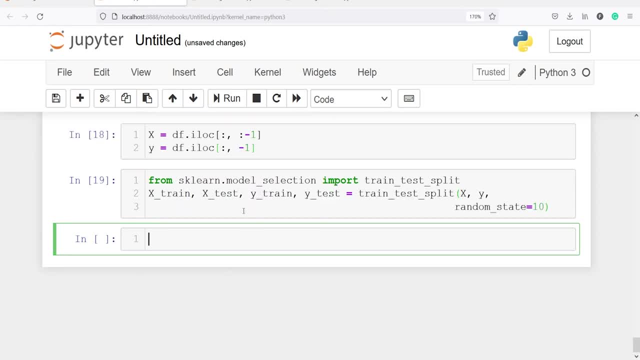 let's execute our code. we have split our data set into training and testing. now we are going to put our code into training and testing. now we are going to put our code into training and testing to import the ridge regression. so let's import from sklearn dot linear model: import ridge. 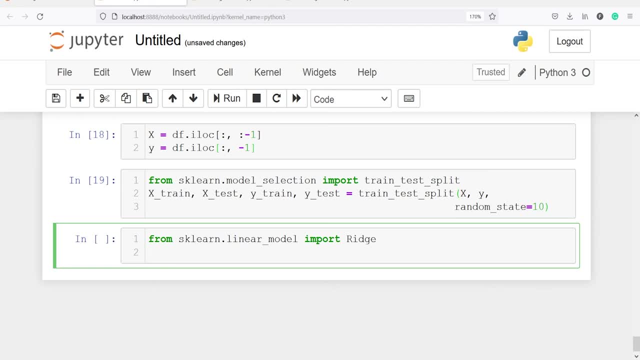 now we are going to make the object of this class ridge. i will write: ridge is equal to ridge, and in this we will pass one parameter, alpha, which is the penalty term, lambda alpha, and here i'm going to put the value as 0.5. you can put any number here, between 0 and 1 or 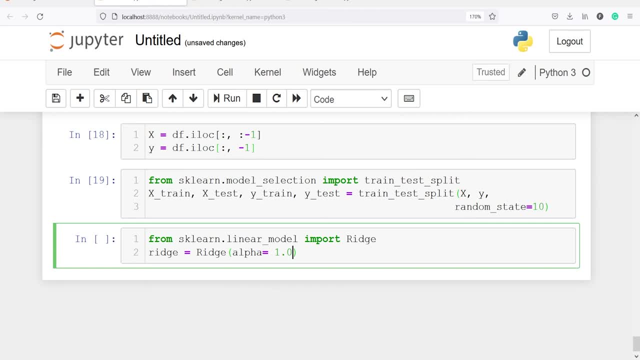 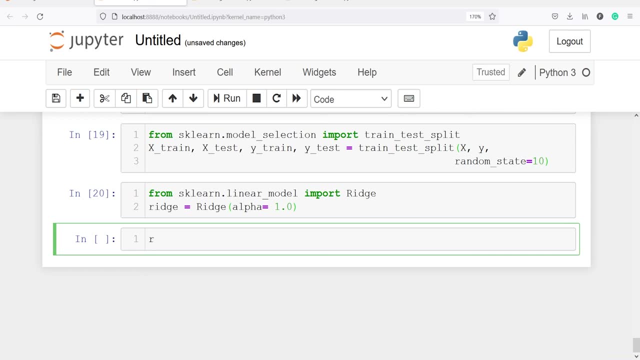 let's say i will put 1, so i will write 1.0 here. let's execute. now i'm going to fit it, so i will write ridge, dot, fit, and i'm going to fit it on x train and y train. let's execute our code. 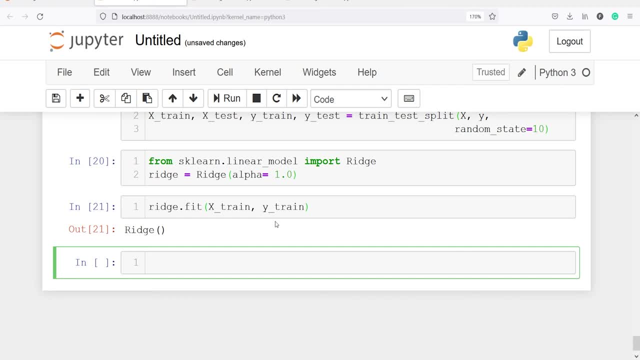 so i have fit this ridge regression on this x train and y train. next i will make prediction and save in a new variable y underscore pred and for that. first i will call our object ridge and from this i will call the method predict. and we want to make prediction on x test. now let's look. 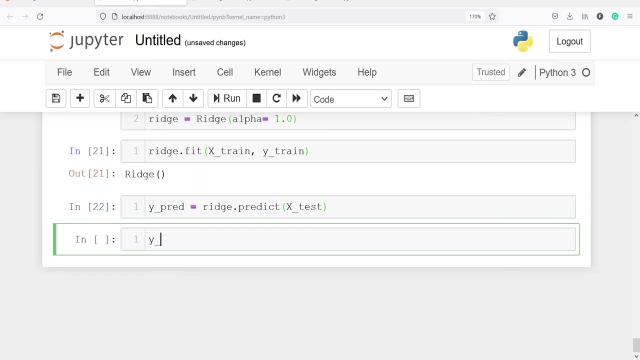 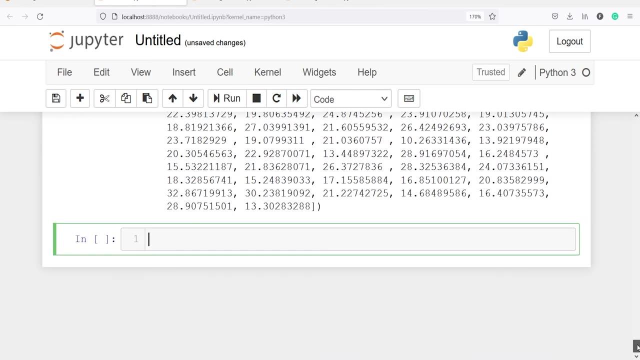 at our predicted values. so i will write y underscore pred here in the output you can see these are the predicted values of gradient prices of our house. now we are going to print this slope and intercept for our model. first we will print this flowpoint five одном. 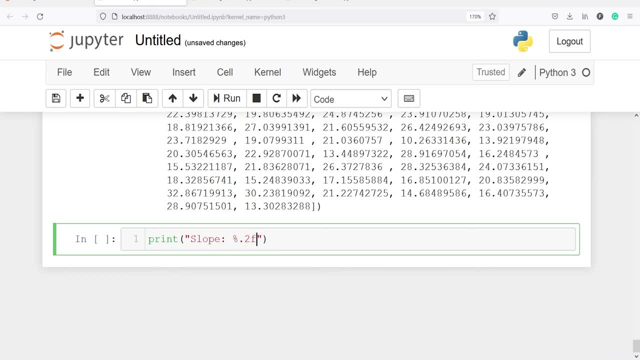 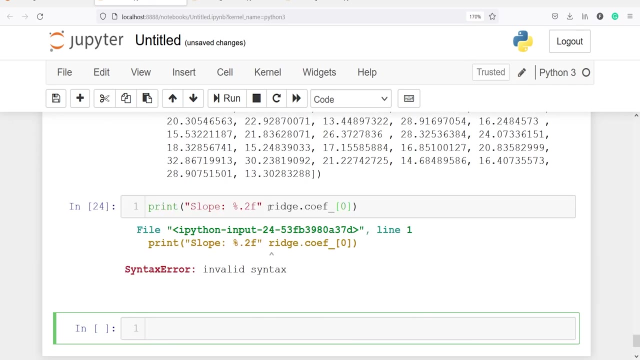 print: slope percentage dot to f. 2f means we want to round it off to two decimals. only then we will call the rich and we will get slope. and slope is present in coefficient underscore and the index number is 0. so we got here. I have to write percentage. 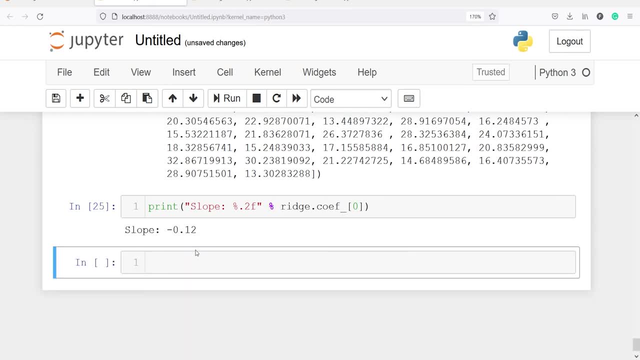 now you will see we got the slope here. our slope is negative, 0.12, and let's also print the intercept. print intercept percentage, dot 2f, because we want to print it to digit. so then I will call ridge and to get intercept we will. 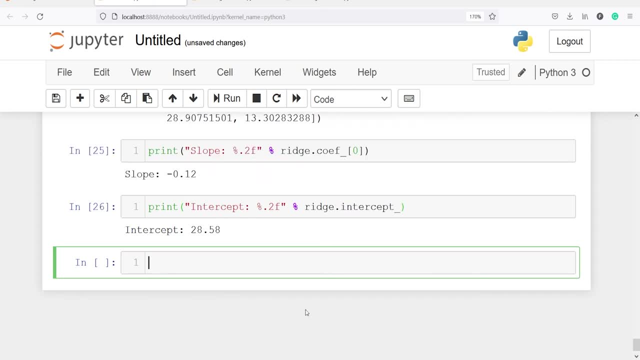 call intercept underscore and here you will see the intercept is twenty eight point five eight here. next we will evaluate our model using the evaluation matrix from sklearn dot metrics. import- mean square error. we are going to get the mean square error and that is falta. input has a ∞M mean square error. 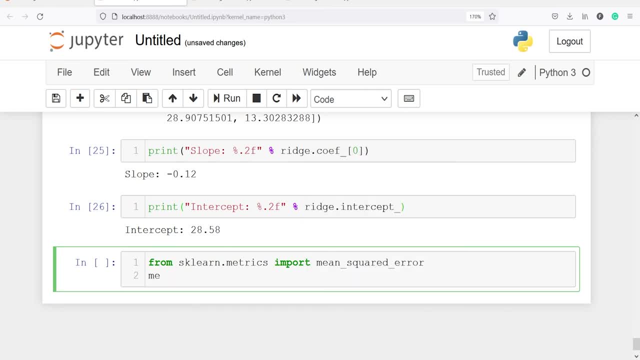 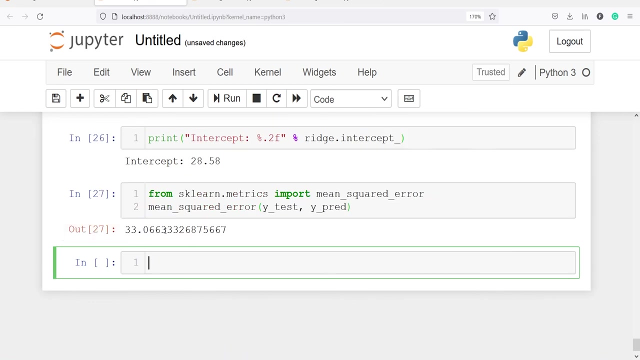 MSE. I will call this mean square error and then I will pass our y test and y bread here. in the output you will see that we got the mean square error as 33. we can also get the root mean square error, that is RMSE. RMSE is nothing but the square root of MSE. so from 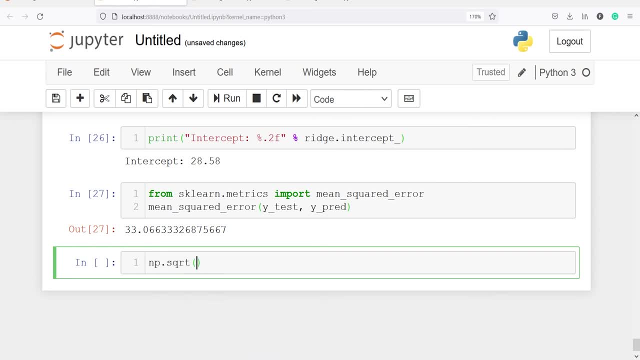 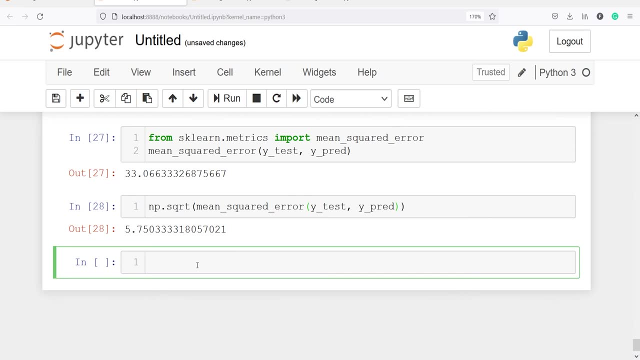 numpy, I will call the matter square root and inside this I will just copy this code from here and paste it here and you can see that we got the square root, that is the RMSE, and RMSE is 5. we can also get the R squared, so for that I will write: print R squared and 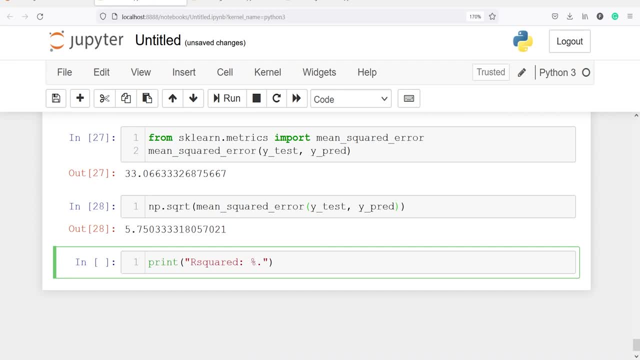 this will also be in two digits, two decimal places, 2f percentage, and it is present in score. so I will call score and I have to pass x test and y test. so our R squared is 0.67. we can, you know, also change the value of this parameter. 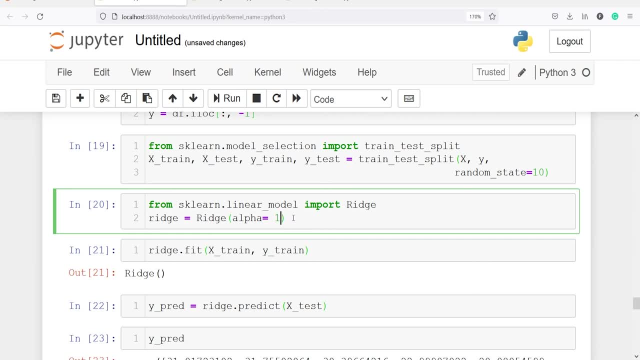 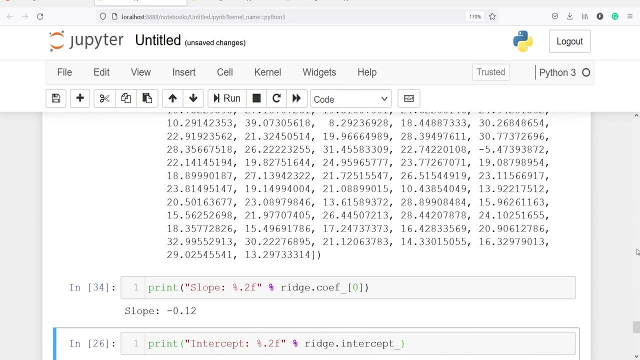 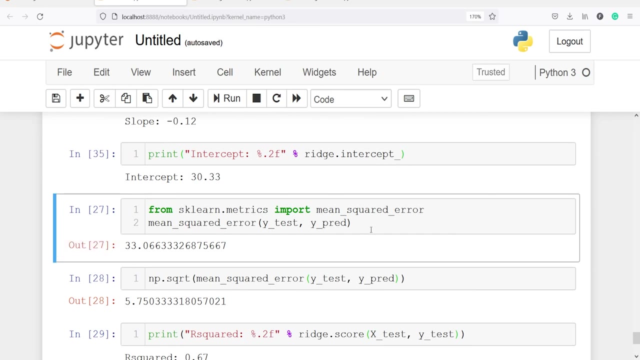 alpha. if I make it, let's say 0.5.. And if I run this again, I will run each and every line. so now let's see if this MSE changes or not. I will just execute. so now MSE has come down to 32, RMSE is same, and let's also 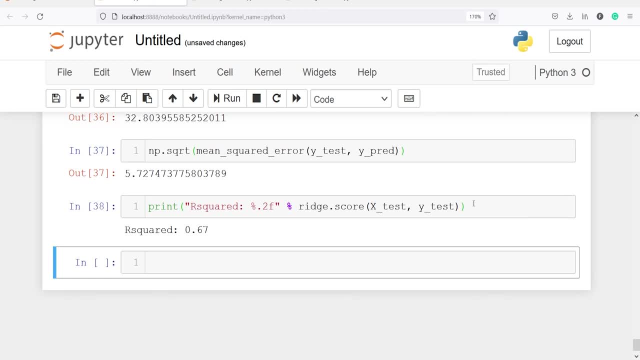 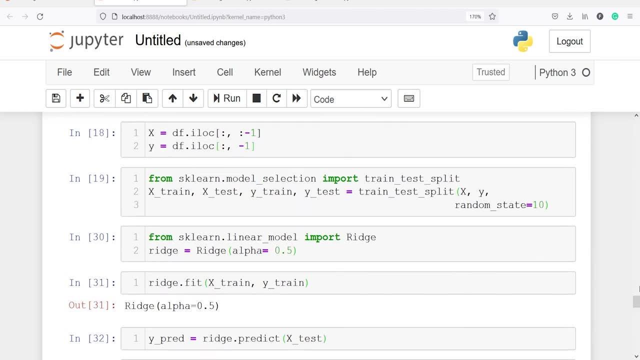 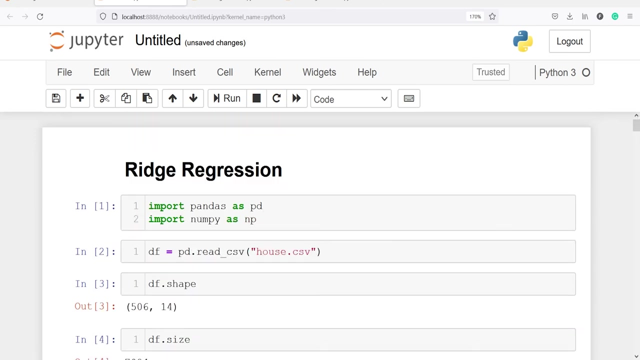 check if R squared changes or not, so R squared also remains same, so you can play around with this parameter alpha. This is how you can develop your retrogression model in python. I hope you enjoyed this video. if you like my video, please subscribe to my channel. thank you for watching.